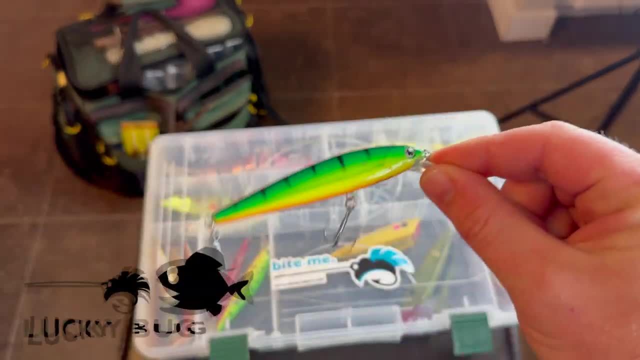 we're going to be using this F-bomb from Lucky Bug Lures, a nice noisy fish hook for pike or walleye, And step two is select your line. For this example, we're going to be using this nice. 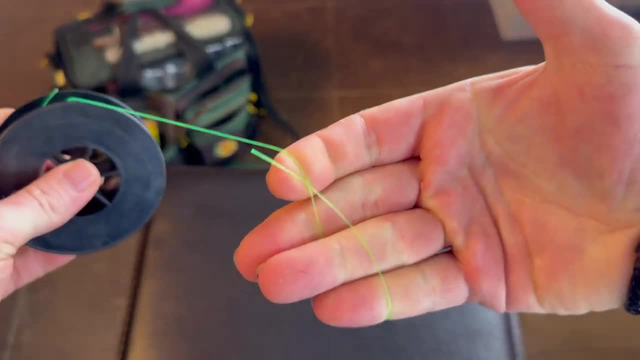 bright green monofilament. I think it's a 25 pound test line, but we're going to be using this bright green monofilament. I think it's a 25 pound test line, but we're going to be using this bright green monofilament. I think it's a 25 pound test line, but we're going to be. 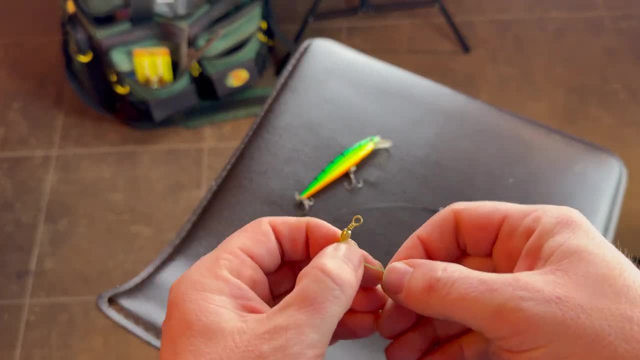 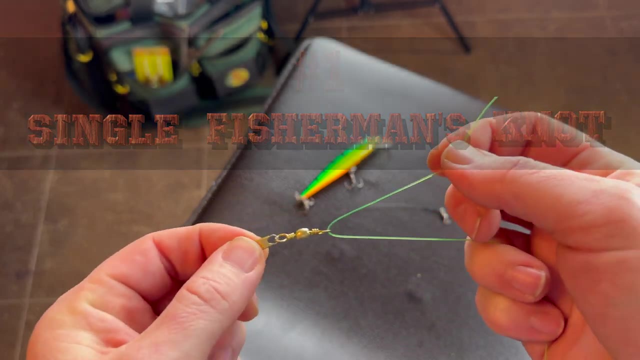 using this, just so it's easy to see on camera. all right, so the first knot we're going to learn is something called the single fisherman's knot, probably the most common knot on the water. chances are you're using it already. the knot is the exact same whether you're tying off to a swivel. 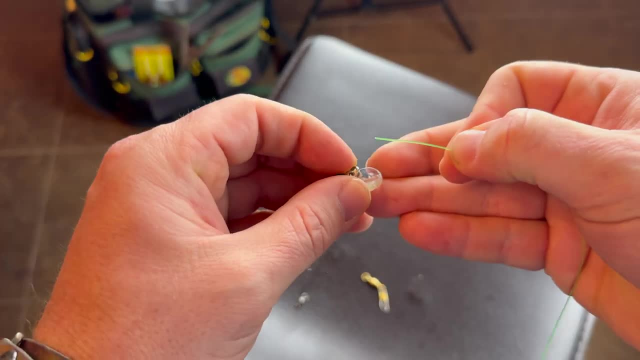 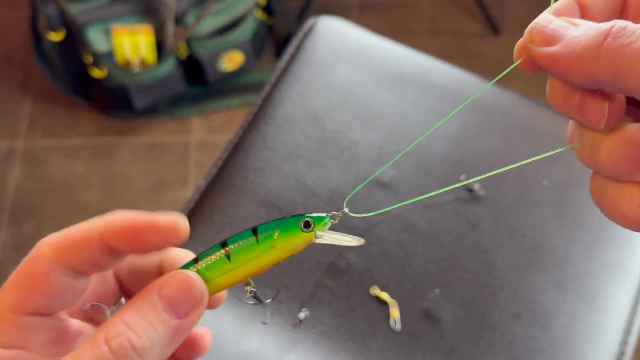 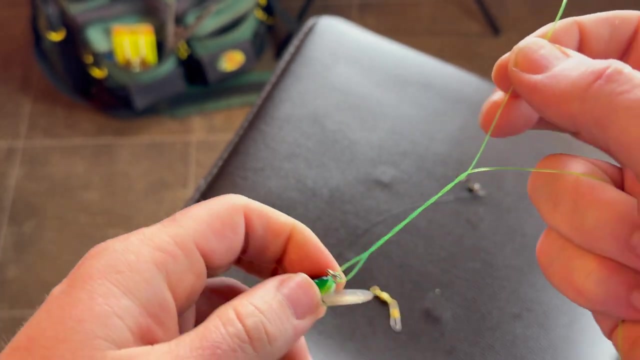 or tying off to a leader, or if you're tying off directly to the fish hook itself. in our case, we're going to tie off directly to this crankbait, so it's easier to see. the next thing you're going to do is swivel the fish hook or the leader or whatever you're tying off to, to get these little. 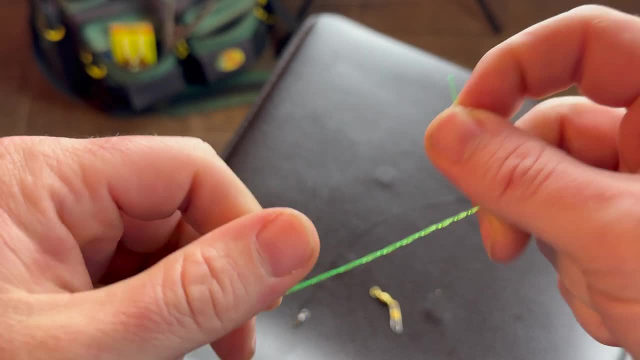 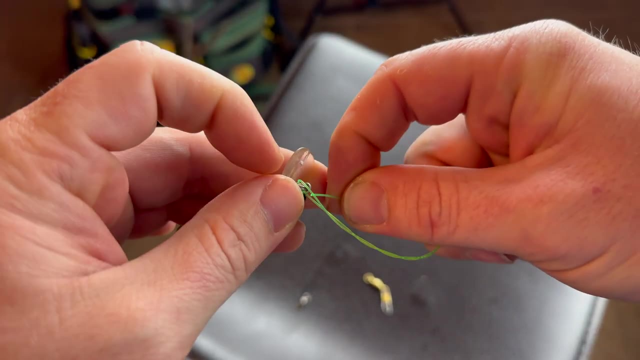 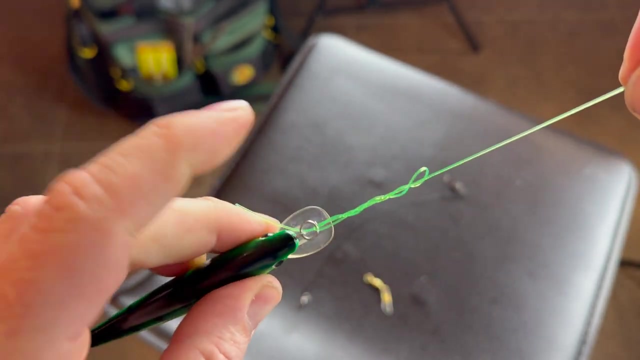 twists in the line. we're going to use these twists to help us build strength. seven or eight twists is usually good. and then you take the leading end of your line and you put it directly through that bottom loop. okay, pull it tight, dress your knot. don't forget to trim your excess, clean your 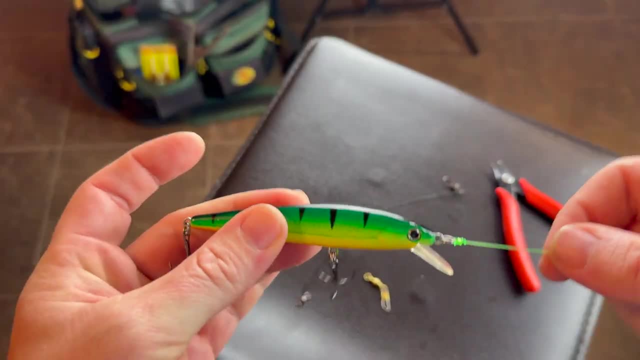 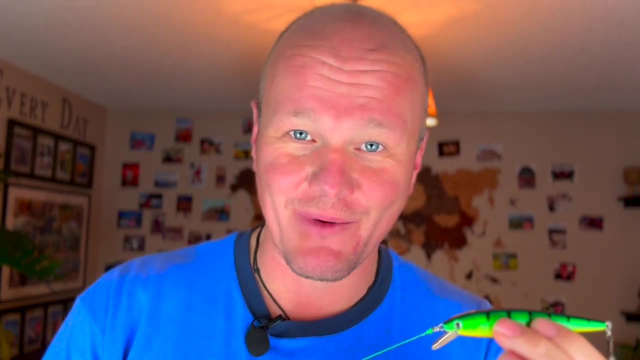 knot and then you're good to go. and there you have it: a single fisherman's knot ready to go, very, very strong, very durable knot. if you can master that knot, you're going to have absolutely no trouble whatsoever with the second one. however, before we get that far, let me just say this: if you're a hunter or a fisherman or a 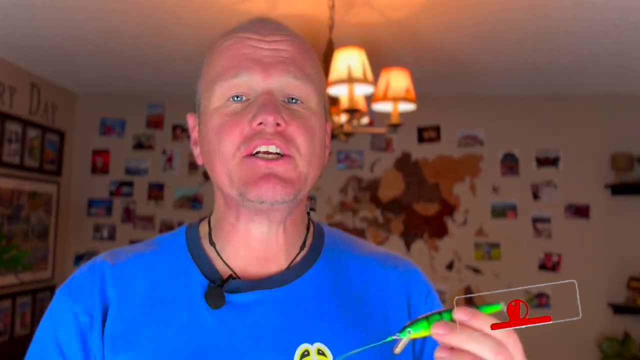 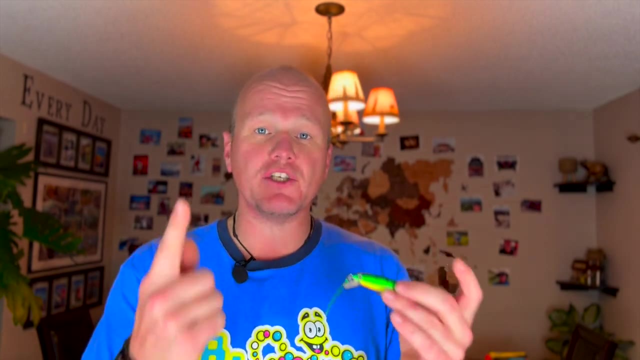 fisherwoman or if you're just passionate about the outdoors like we are, consider clicking that subscribe button down below. i know it takes less than half a second, but it means the world to us as we're trying to grow our channel so that we have the opportunity to do more product reviews. 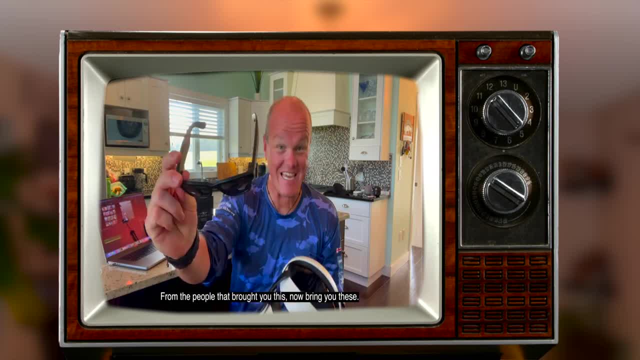 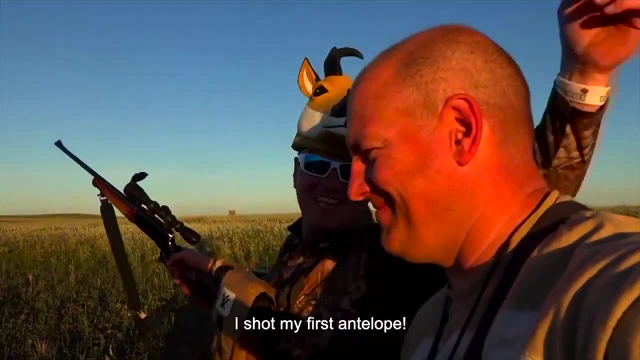 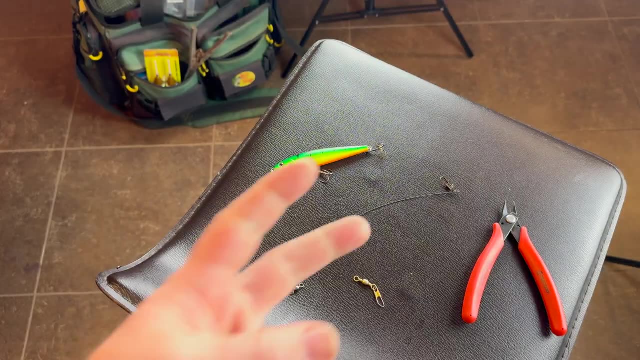 the people that brought you this now. now, bring you these now. we're taking them fishing more giveaways. do more full-length feature films. if you haven't had a chance to check out our library yet, head on over, because i guarantee you're going to find something that you're going to like. now here's knot number two. okay, guys, knot.